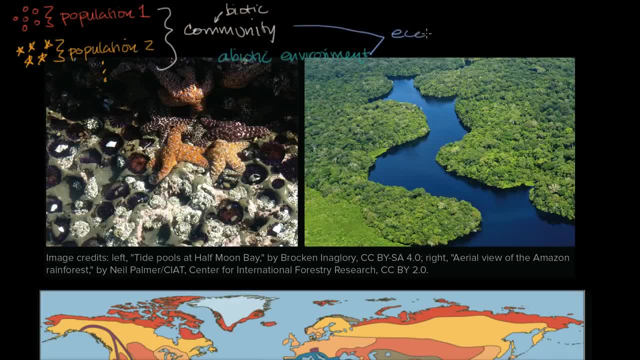 You put all of these things together and then you get your ecosystem, Your ecosystem once again. it could be a very small region, it could be a very large region, but it's made up of all the living things, the biotic factors and the non-living things. 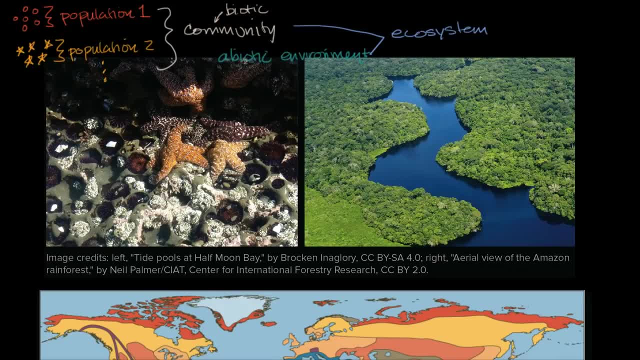 the abiotic factors. Now, what we're gonna think about in this video is just the types of ecosystems that you might have. Think a little bit about it And also begin to think about how the the different, different factors interact with each other. 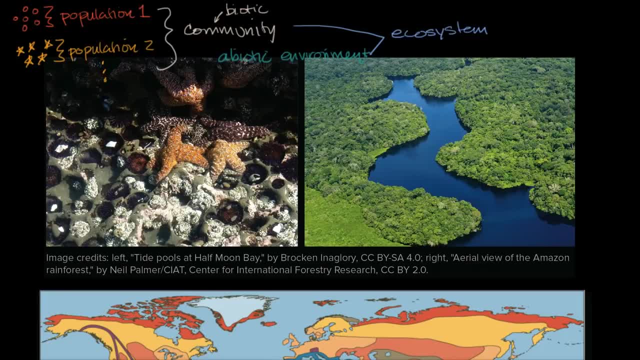 how there's a conservation of matter, where, within an ecosystem, matter tends to go from one form to another. You also have a flow of energy. Energy tends to enter an ecosystem in form of light, and that energy gets transferred from one organism to another. 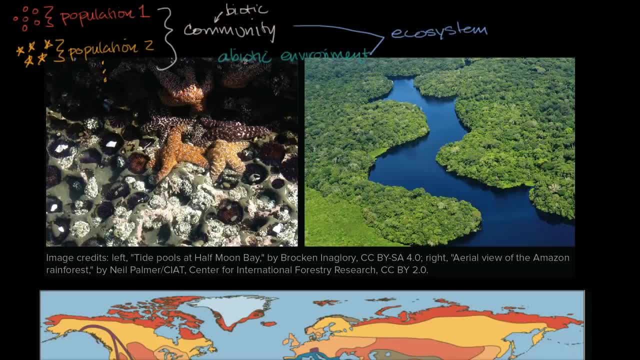 and sometimes even involving the non-living things eventually becoming getting turned into actual heat. Now, in terms of the types of ecosystems I already mentioned, there's a lot of variety there. This right here is a picture of a tide pool at Half Moon Bay, not too far from where I live. 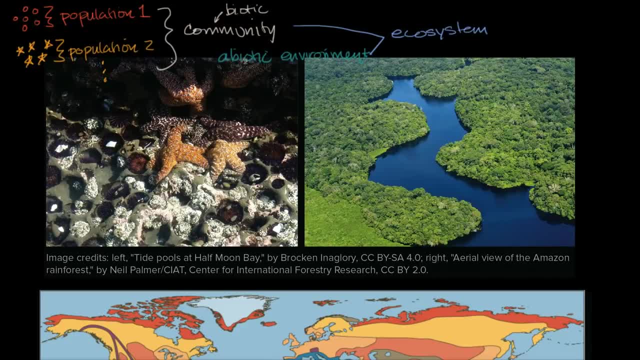 I've actually been to the tide pools at Half Moon Bay And you could consider one particular tide pool. both the abiotic factors, the water and the rock there, as well as the biotic factors, the starfish, the sea anemones. 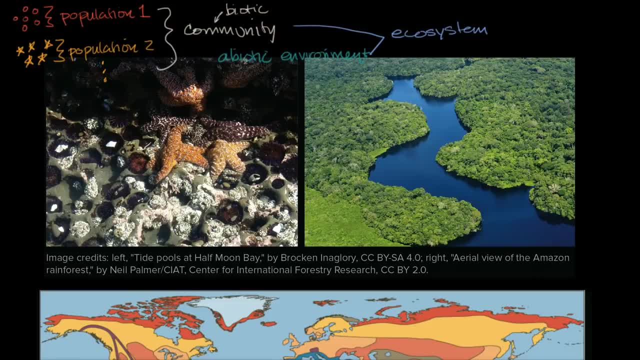 and whatever else might be living there. Those combined, that could be an ecosystem. You might say that the entire beach is an ecosystem. You might say that the entire region is an ecosystem. Once again, it depends on how much you wanna zoom in. 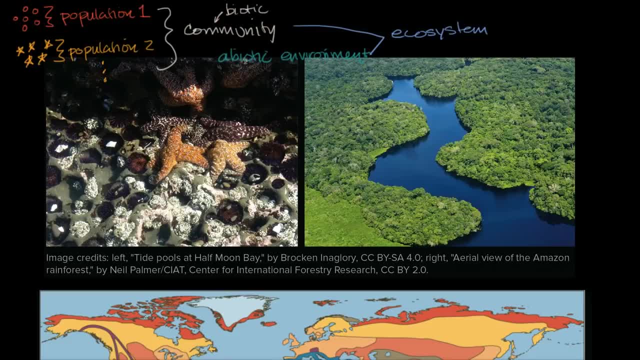 or how much you wanna zoom out, And you can zoom out a good bit. This rainforest right over here, this is the Amazon rainforest. you can consider the whole rainforest an ecosystem. Or maybe you just wanna study. maybe you just wanna study what's happening. 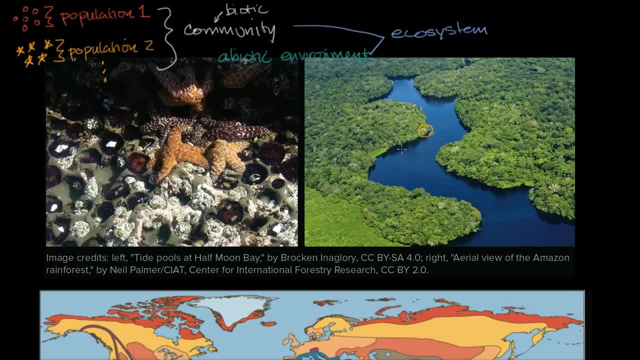 in this exact region right over there. You could also consider that an ecosystem. You could consider what's happening in the river itself an ecosystem, or maybe one part of that river, And, as you notice, I'm talking about some ecosystems that are on land and some that are in water. 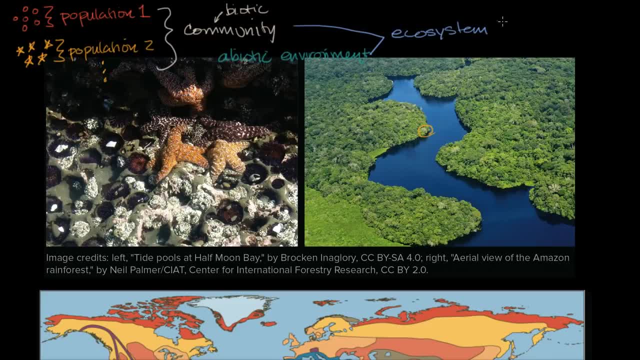 And that is a general way, one way of classifying them, So an ecosystem. you could have it on land, you could have it on near in the water, so we could say it's aquatic, And then even within aquatic you could have ones. 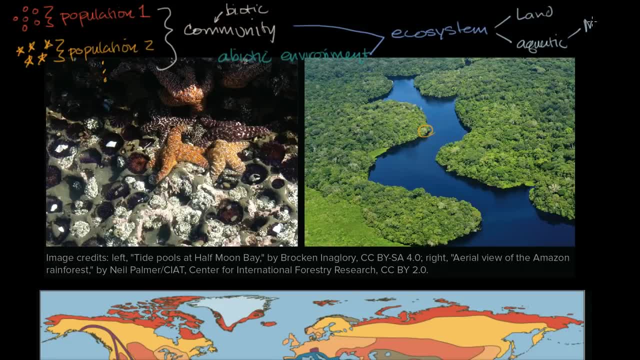 that you have salt water or partially salty water and these are called marine And the main marine ecosystem. we're thinking about the oceans and things like that. And then you have freshwater ecosystems, Like if you are in the upper Amazon, that is freshwater, that is flowing. 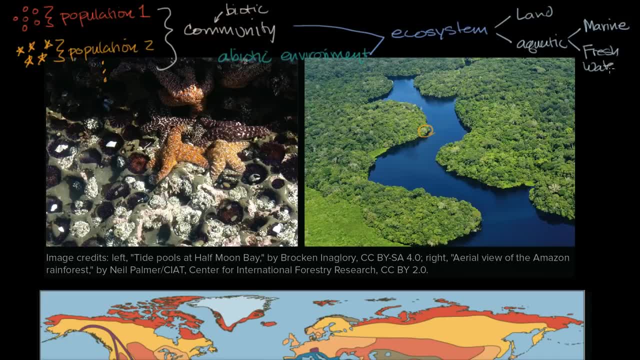 So we could say fresh, freshwater, non-salty water And even though it looks like rivers are big and there's a lot of freshwater around us, obviously we need freshwater to live. most of the aquatic ecosystems are marine, are not involved freshwater. 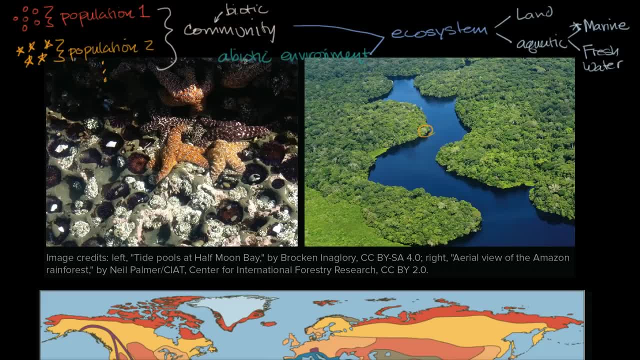 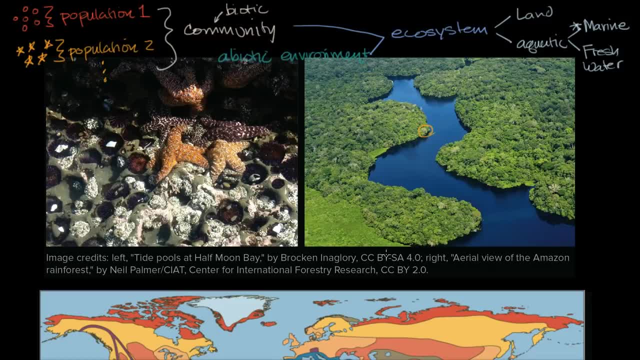 you could view parts of your body as an ecosystem. you could look at just a fraction of- if this is my hand right over here, you could just take a little square there and you could consider that an ecosystem And you can think about the different bacteria that are there. 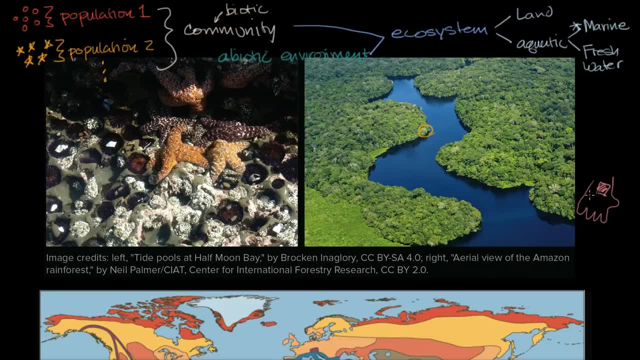 the other types of microorganisms that are there and how they're interacting with the non-living things- the air, how they're interacting with the oil on your skin, with the dead skin cells, and also how they're interacting with the living skin cells. 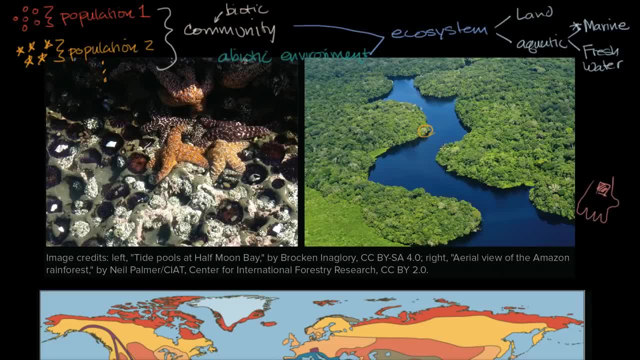 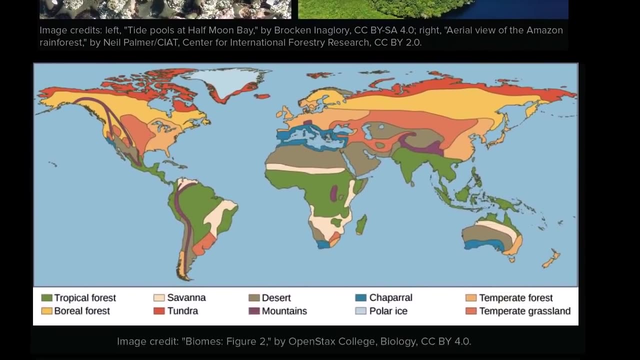 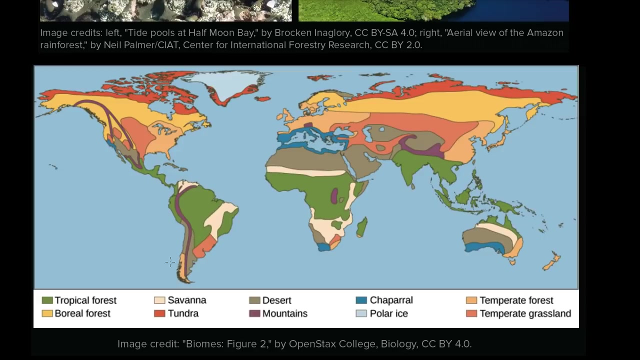 and you yourself, Since we're focused on how we can classify ecosystems. one thing that's often done is classifying land ecosystems into various categories, And right over here we have depicted the major types of land ecosystems on our planet and where you might find them. 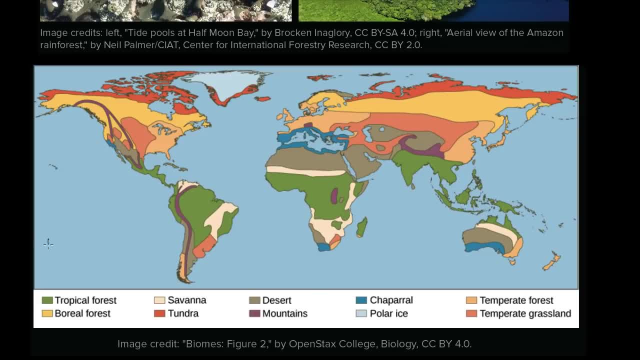 And these different types of land ecosystems. these are called biomes. biomes And, as you can see from this, this is the Amazon diagram tropical forest. You could find it right over here. this is the Amazon rainforest. You can find it in Africa. 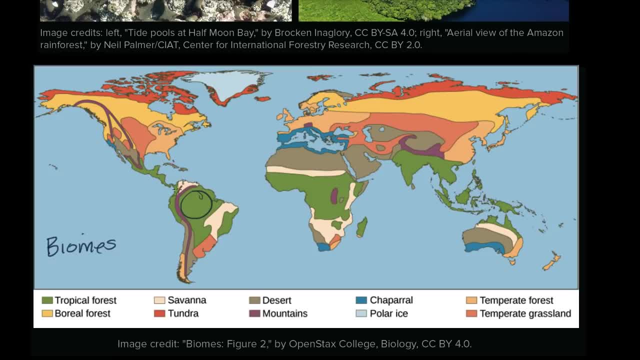 you can find it in Southeast Asia. you can find it in Central and even Southern North America. You have boreal forests which you'll find in more northern latitudes: savanna, desert, tundra, chaparral, polarized. 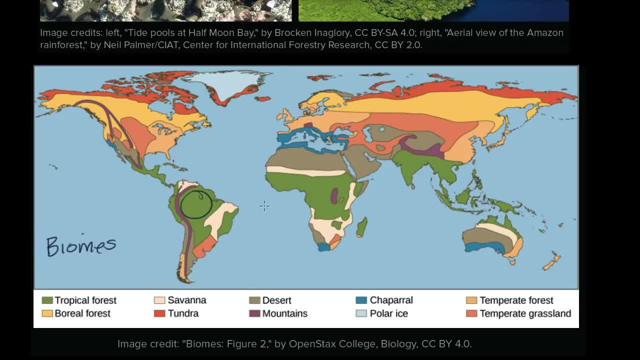 temperate forests, temperate grasslands, And these are just helpful for thinking about roughly the types of ecosystem or ecosystems we would find in those regions, And it's typically most determined by temperature, moisture, the climate- actually the climate- and the terrain.